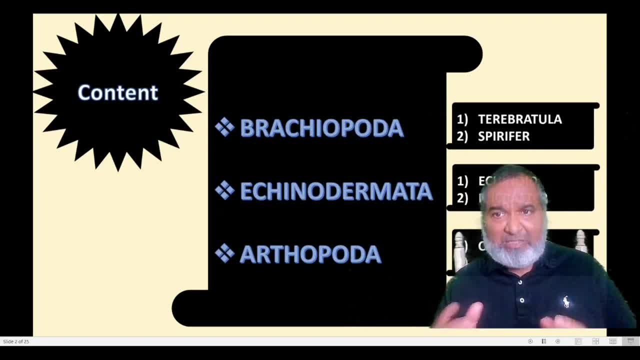 and micraster we have a fossil. So these six particular specimens we are going to study from three different phylums. In earlier, first practical of paleontology we have said that we have seen the phylum mollusca and in that class, lamellibranch, harka unio pectin. we 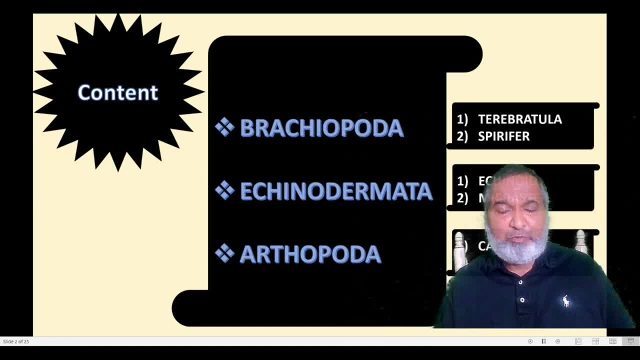 have seen. Then in gastropoda we have class gastropoda. we have seen turritella and fisa and third one, class cephalopoda. From there we have seen Nautilus and ceratite. Now these are again six In this practical we are going to see. let us start the phylum brachiopoda. 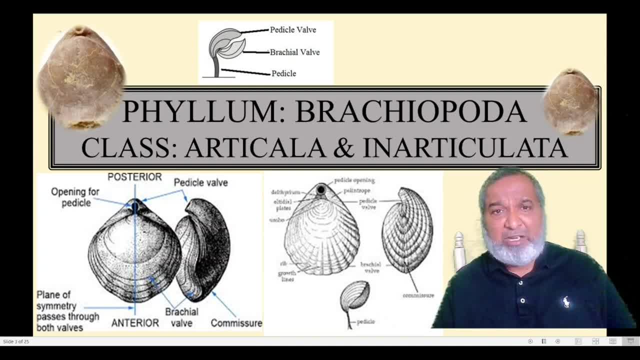 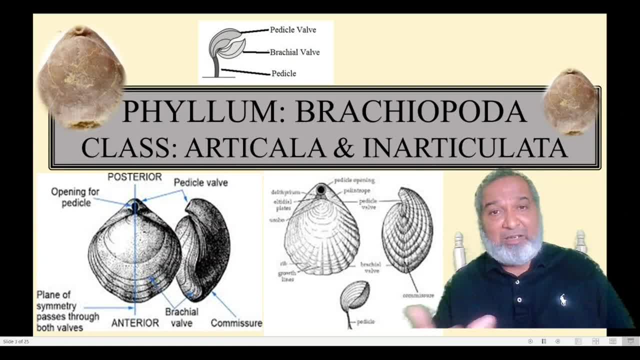 so that spelling mistake is there. So I tried. but so many pipitis I am preparing at one a time and simultaneously I am going for videos editing and all that. So that will be a minor error. So human error is there, So it will be there and you are going to see that. So 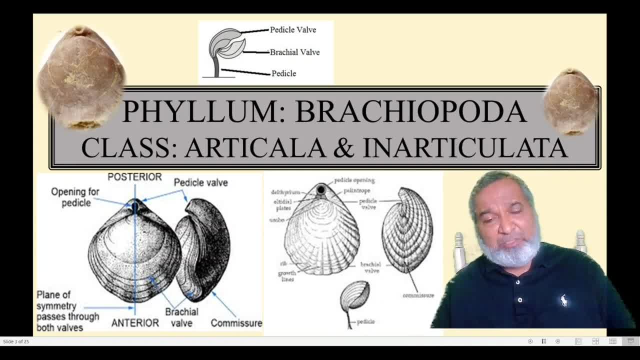 I appologized for that particular spelling mistake, that articulata, But in articulata inarticulator is there. but now from the whatever we are going to see the specimen today, both are from the articulator class. first we'll see the morphology. what are the characters of brachiopoda? 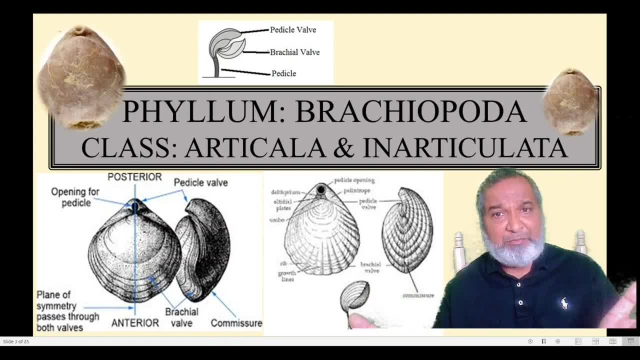 a brachiopoda, which is there. it contains two shells. yes, both shell. in case of lamellar branch, there also we have two shells, but in lamellar branch if you join your two hands they're exactly similar: shell or shells are shells are there. that is a wall we called as left wall and right wall. 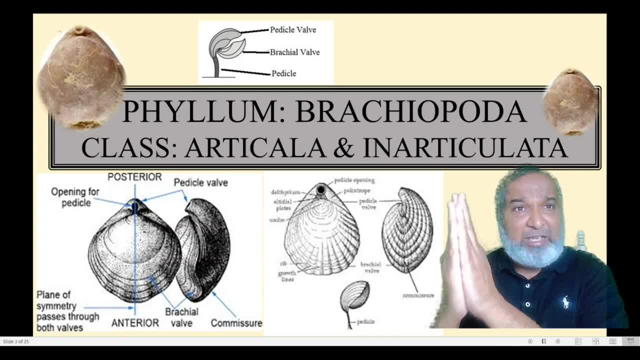 they're exactly matched. so, lamellar branch, they are equivalent. but in case of brachiopoda, you can see whatever. we have shown you the diagram. see now, this is a perfect diagram. so if you just bend it out, here we have the what we have. the pedicle opening is there. that is the. 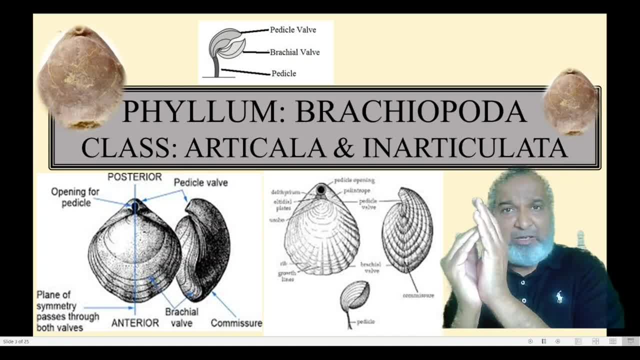 humbo is there and this is one wall is bigger, one wall is smaller. and wherever we have the pedicle opening is there. that wall is called as pedicle wall here we have been shown here. this is the wall where we have the pedicle is present. it is. 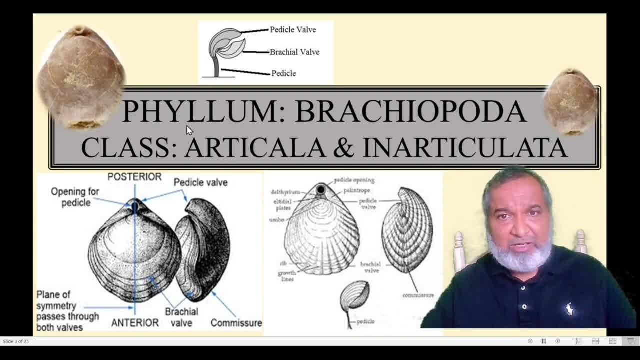 a bigger one. so here we have the bigger wall which is here. yes, so everywhere we are shown we have a fossilized specimen and these are the specimen from the department we have been shown. the photo photographs i must thanks from for my lab assistant and, um, my student uh non background from the geology NCC especially they have taken the photograph. 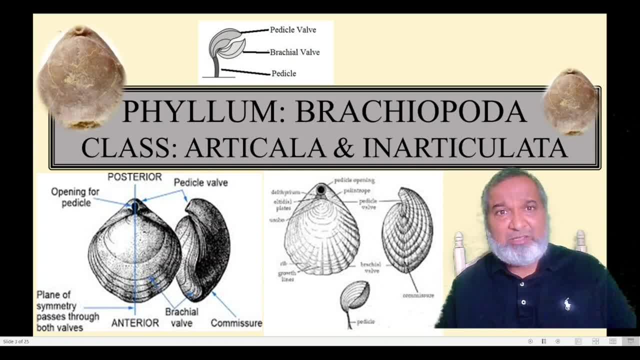 and my lab has and uh, Mrs Shaheen, he has uh shown them the what are? the specimens are there and they are taking the uh professional uh with the camera. they are taking the photographs and they send me in a US. so i'm preparing this video sitting in a US and you're going to see, you know. 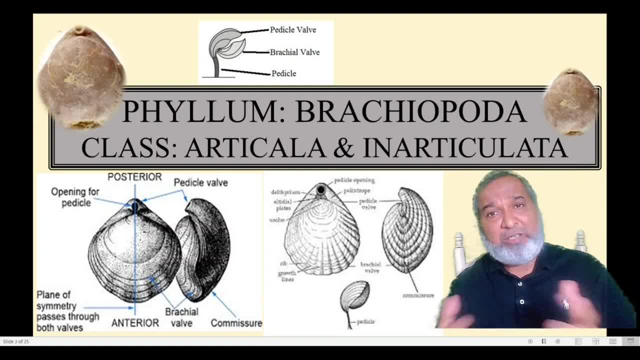 shortly when i'm going to upload all my videos from in a US and you're going to see you know shortly when i'm going to upload all my videos from. i am uploading now, so when i once, the college will start at once. i joining in the month of. 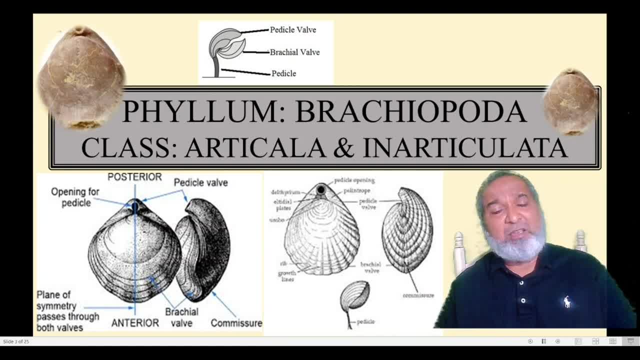 december or jan i am going to join this department and at that time, whenever i have the free time, i will go again, going to reshoot this one with the chalk and board so that you can get, and at that time you can get the specimen in hand and see the details again in a new videos will be uploaded, so 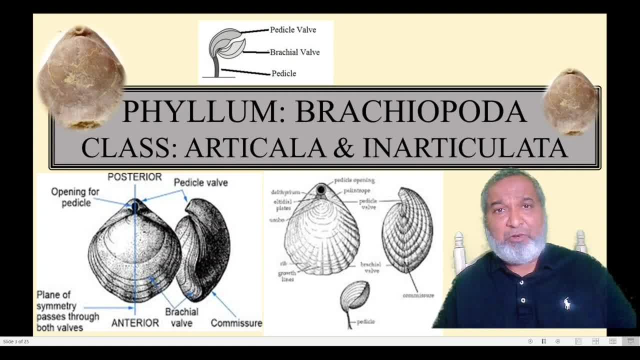 that we can get the more clear pictures for about all whatever practicals which are going to tell. now, this is the practical where we have the brachiopoda you are going to see in this, one wall is bigger, one is small, so in equal. yes, this is the first important term regarding brachiopoda. 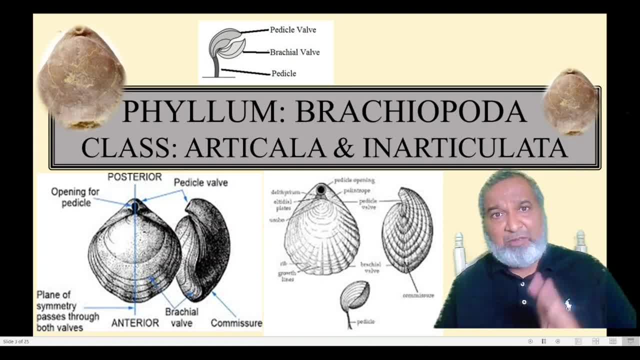 is, walls are in equal. but if you bring it the particular wall and if you draw a vertical line- yes, in this particular diagram you can see now here i have drawn a vertical line here. so the shell is exactly going to divide. so it is equilateral. but in case of lambly branch, if you 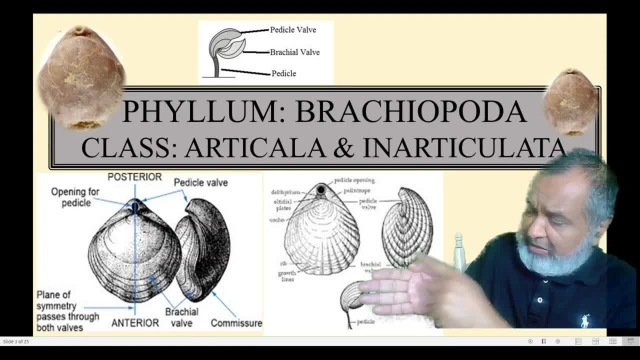 make out and if you want to draw a line from number one side, but this side we don't have, so asymmetrical is there. so it is in equilateral over there, but here, in the case of brachiopoda, the, whatever the shells are there, it is the equilateral. 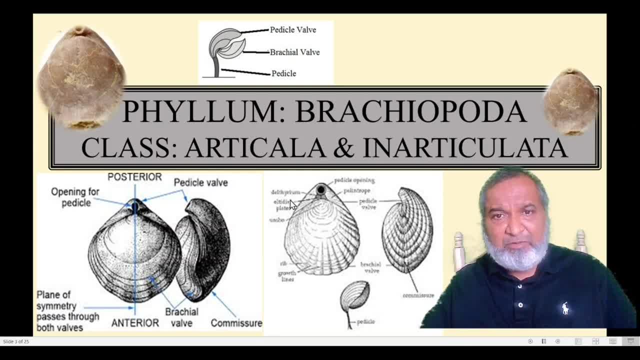 and here we have the hinge line. is there? yes, so that will be the part you can going to see the various parts to then this commisuture plane is there, you can see. that will be shown. yes, commisuture is there. so, whichever the small is there brachial wall. whichever the bigger one is, 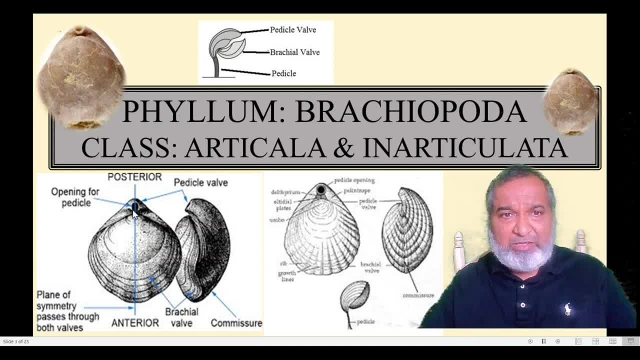 there, that is the pedicle wall, and wherever the ambo is there, yes, that ambo is the posterior side. this is your opposite- is the anterior side. yes, so there in the lambly branch, what is happening? dorsal side, ventral side, wherever it is pointing, it is anterior side. so that is there. so that is. 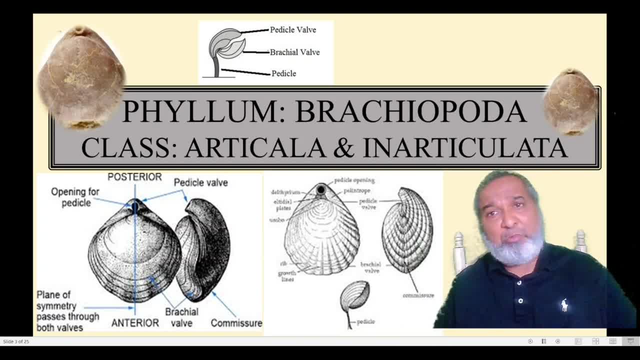 also a difference between the lambly branch and brachiopoda. so i'm going to make a separate video on similarities and dissimilarities between the brachiopoda and lambly branch. that also we are i'm planning now, so work is good, so i could. once i finish this one, then i could go to the next one. 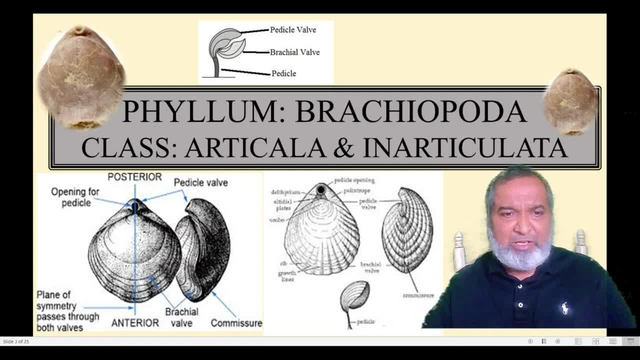 for that particular part also and that you are going to see in a shortly, but today we are going to see this one. this is the. what we have is the towards the posterior side, the wall will be there and opening and closing from the lower side. from the anterior side, they are closing and opening. 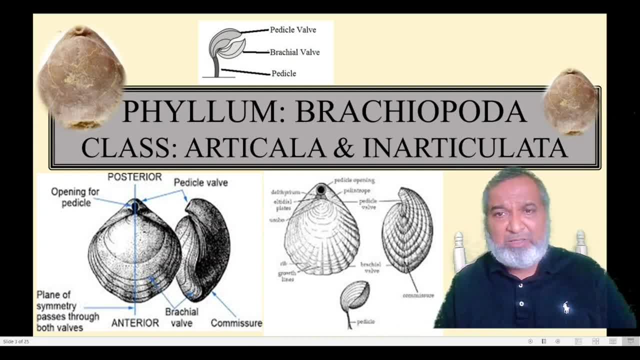 muscle scar will be there, which will be going to help into this, and that will be the part will be there and wherever the pedicle opening is there, from this part the muscles comes out and the the leaving. when the animal is leaving, the muscles comes out and it will attach to the rock bottom. 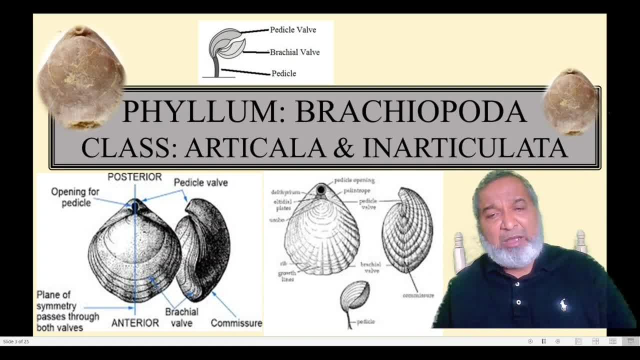 pedicle opening. but that pedicle opening will be covered, uh, by a plate, deltidium plates, so that will be there. yes, that is a 10 calcareous plates will be there. that is going to cover the body. this is the thickness, if you see the shell thickness. this is the height of the shell. 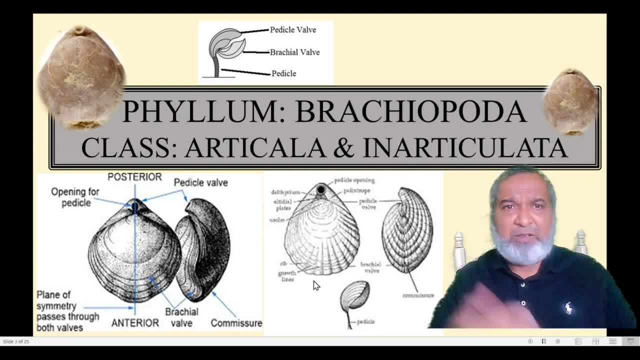 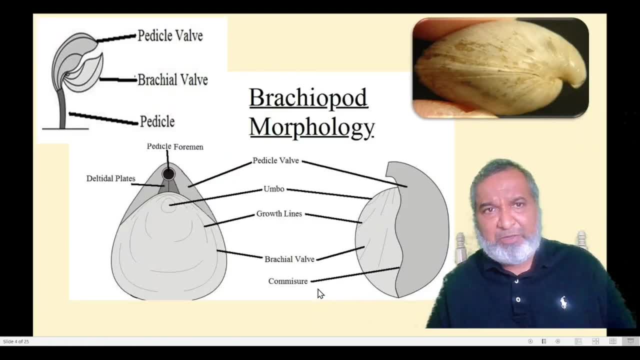 and this is the length. yes, this is length. these are the things. when we are going to see the similarities and dissimilarities in that part, we are going to have that video again. you can see pedicle opening brachial skeleton foramen or pedicle opening deltidal plates are there, these plates are going. 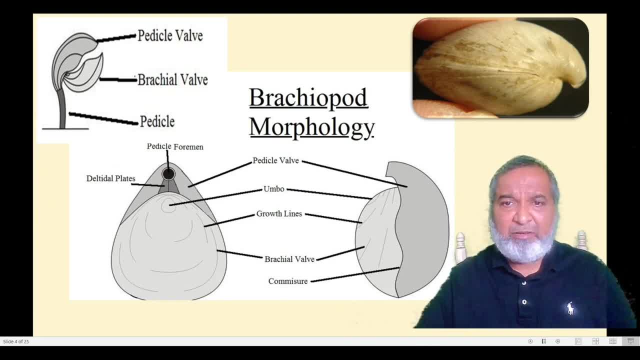 to cover. uh, whatever we have, the foramens are there. umbo is a prominent one, yes, elevated portion. umbo growth lines are there? brachial skeleton, the smaller one, homey suture plane, along which the two planes are joined together, and here it is a very good one. fossilized one is there, you can see the comisucher is there. 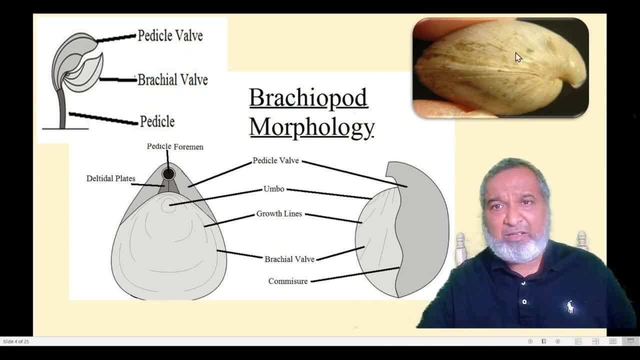 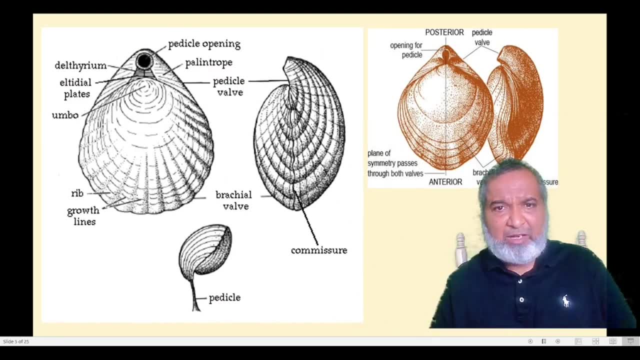 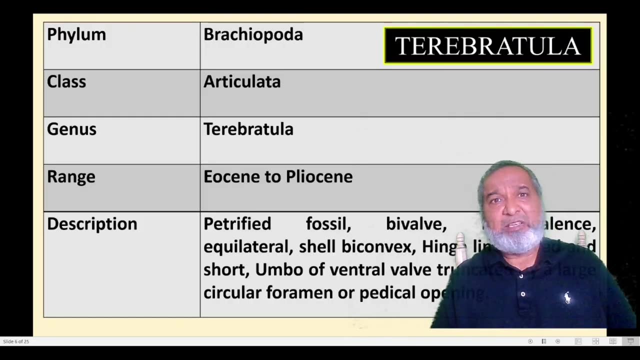 this is the ambo critical opening, yes, and this is what we have- critical wall, and this is the brachial wall. a same diagram, again, i am going to repeat and so that you can get the more visualization in that particular part: yes, come to the next one, description, how you are going to describe what exactly you have. 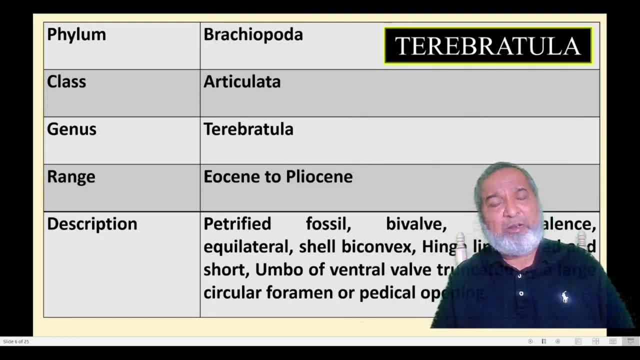 to do it in the practical. this will be given only the theoretical part, which is: this is the whatever we are giving you, this will be. you're going to write in the journal, but in the examination this will be the spotting, is there? so what exactly you have to do in the practical? 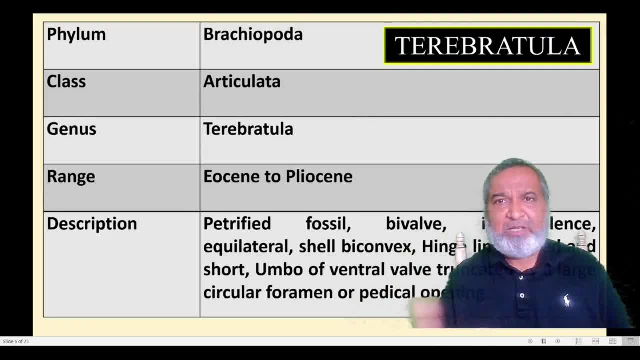 whatever the spot number say now, it will be changed because of our credit system is there? practically also come in a credit system wherever the spot is there. for example, this particular terrible auto is coming at a table number five. so what do you have to write down? you have to. 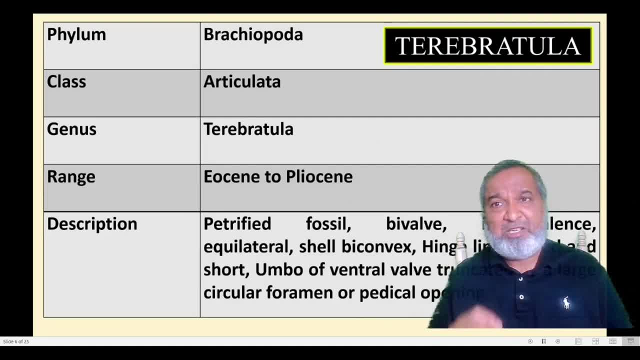 write down the classification: phylum class, genus and range. these things has to be right down. so each one will get the half of marks. yes, if the phylum class will be there, that will be one mark for the classification. half mark will be the genus and half mark will be the range. 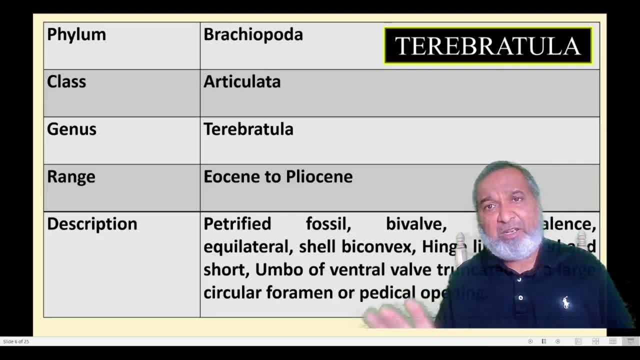 next one. whatever the description is there, it is not required in the examination. we want a neat label diagram. so whatever you know the parts you have to write down, draw the diagram, neat label diagram. so examiner will understood that you have been understood that particular part. so here what we have: the terebratula is phylum brachiopoda. 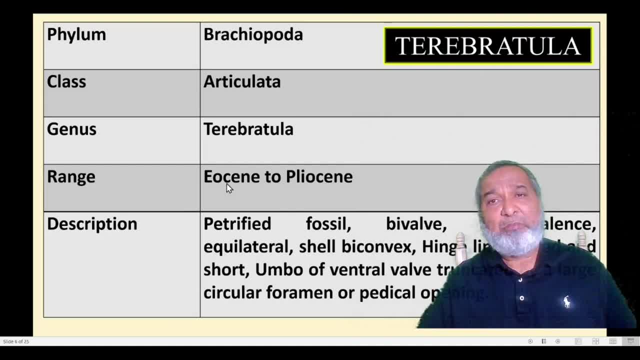 class articulator terebratula genus, and it is from the ranges eosin to hyosin. i told you this is a petrified fossil. it was in equi-valence, that is, in equilateral. that is the in-equivalent. it is written in equal wall in uh. this is the equilateral. shells are biconvex. 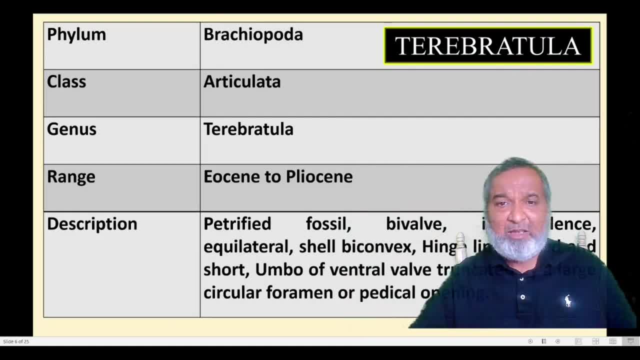 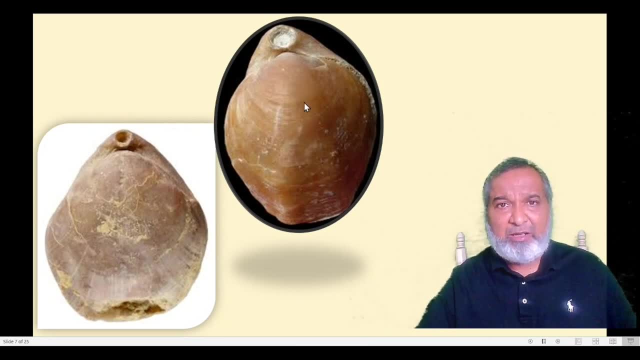 angeline curve, that we are seeing the curvature is there, yes, humble ventral wall truncated by large circular foramen. that is there, that we have shown, and there is a radical opening. is that? yes, this is what we have, the perfect pedicle opening. this is what we have. the brachial wall. 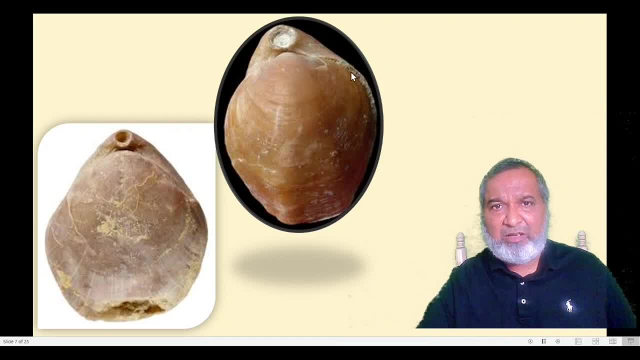 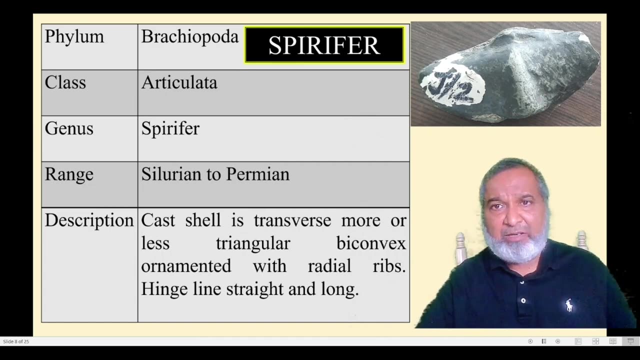 pedicle wall and this is the hinge line. is curvature. ambo will be there. so these are the parts we are shown. the growth line is there, dorsal side, anterior side. next one: we have a cast fossil. this is the cast fossil that now to see it is broken hinge line. 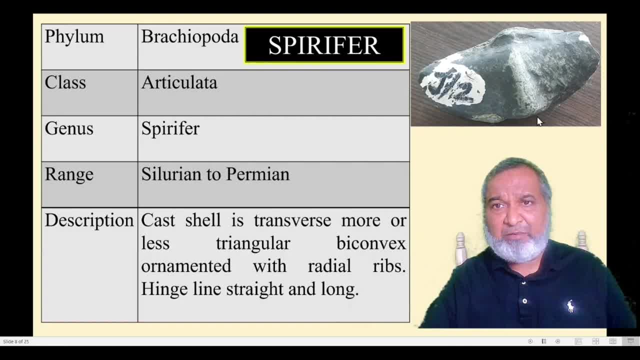 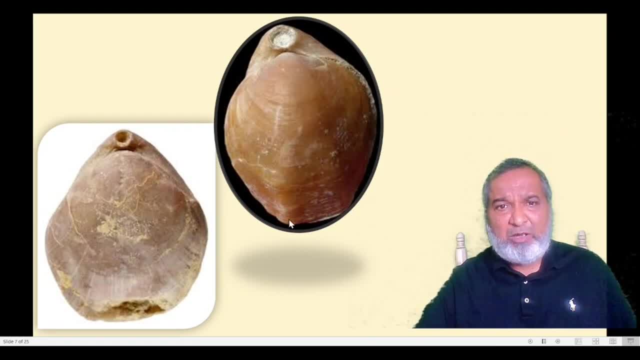 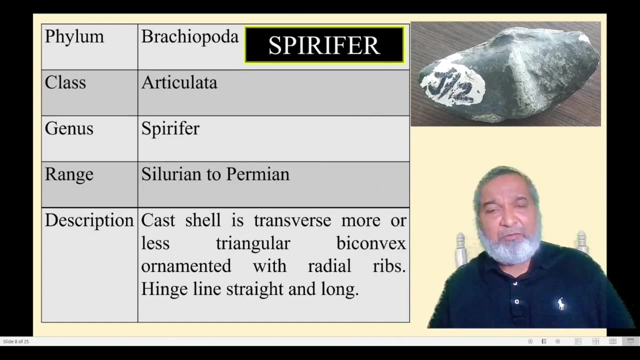 is straight and this particular specimen is somewhat triangular. there also what we have is, if you see this particular part, it is oval or somewhat triangular. so that will be the shape. so that comes under the what we have: the forms of the brachiopods, what will shape, size, orientation. 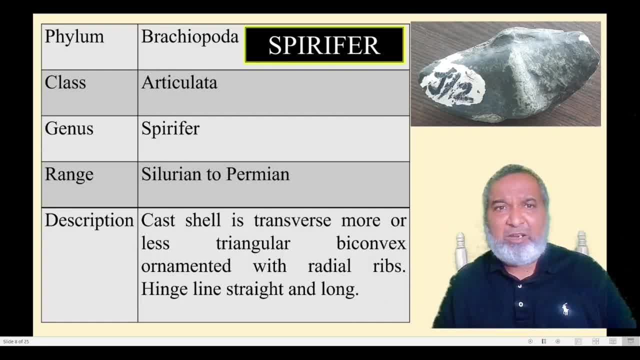 ornamentation is there, but now we don't have to go into the detail. phylum brachiopoda, then, class articulator and genus is peripheral, silurian to permian. silurian to permian is the range of this particular. the spirifer cast shell is there. that i already we have seen. from their diagram you can find out. 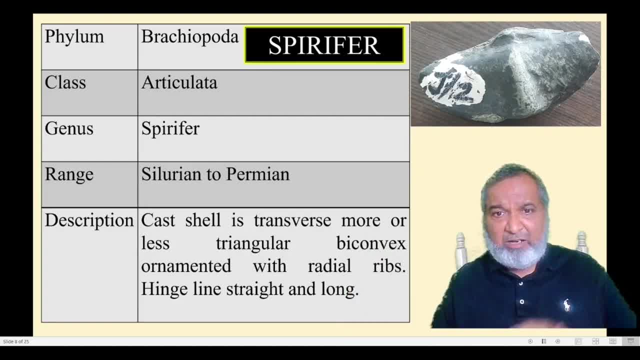 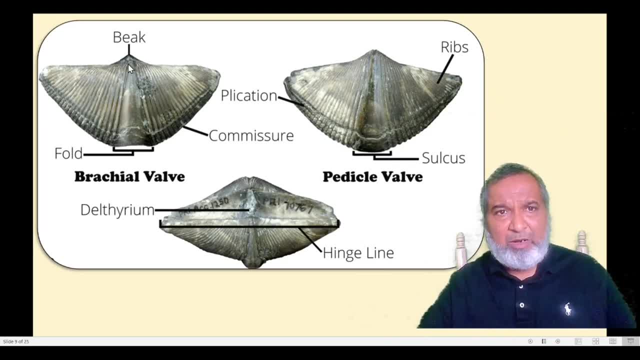 again, it is a biconical. both are the triangle which have been there. hinge line is straight and long. these are the thing which we are going to make out. yes, again, ornamentation, which are there, but we don't have the fossilized one. yes, the ribs, which are there. 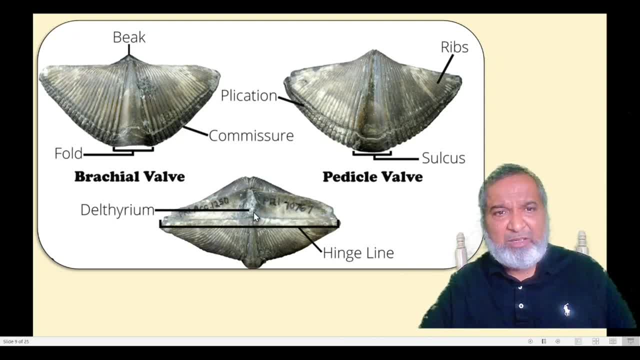 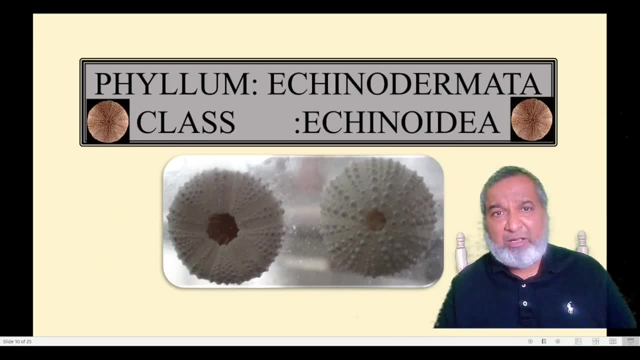 tools: see the hinge line. so delterium. so these are the bivalves dorsal. so all positions we have been taken out. next one: phylum echinoidermata and class echinodermata. this is what we have. the specimen glass model is there because it is a more exoskeleton, is there just if you press it down it. 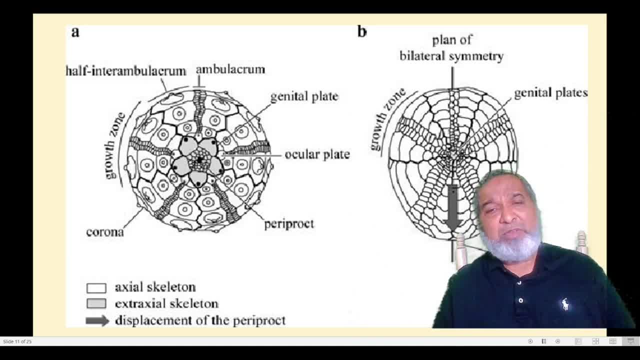 will be broke out, that is, the echinoidermata one. so in this what we have, the body is divided into three parts. first one, the physical body cell, which we have, and then, as the shape of this particular equine edia is there, it will be divided into two categories: regularia and irregular. so a is 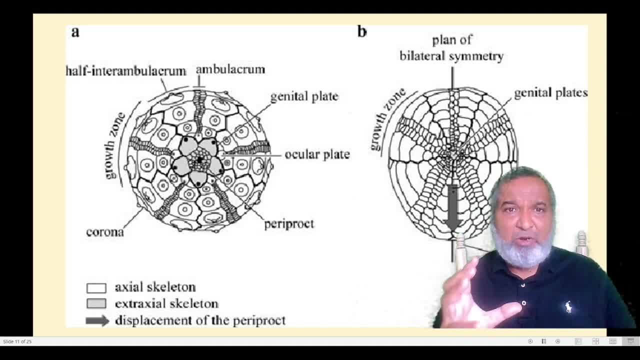 the regularia and b is irregular. now in these two, what we have, the, whatever the body, is that it is composed of three parts: the major part, which is that the corona, then the next one, we have the apical disc and and peristrole. these are the two. 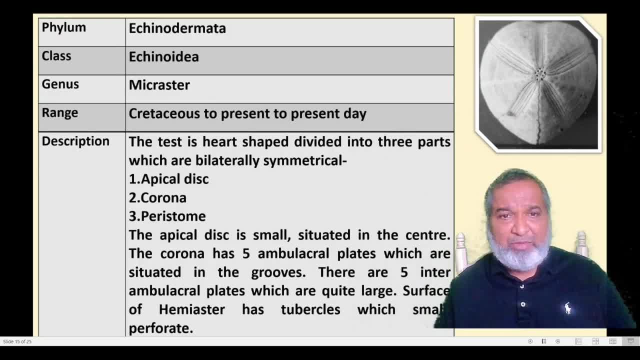 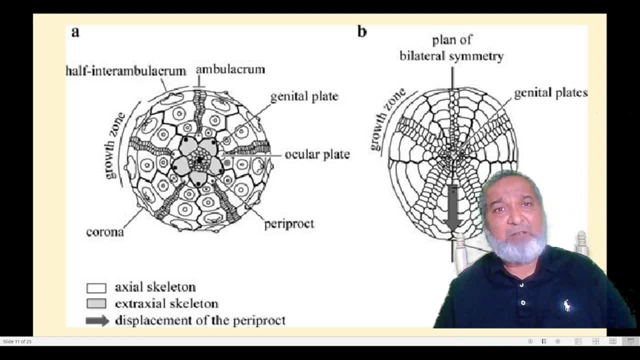 the imaginary line, whether apical, disk and peristome, then this is the centrosymmetry. assume now we will have the axis symmetry. centrosymmetry will be there. then that will be the regular one and second one. if you draw from the center, yes, if you draw from. 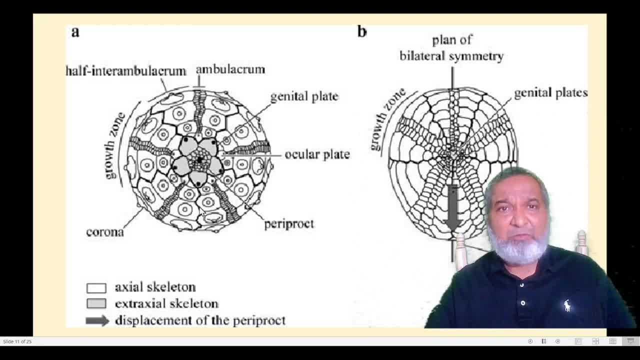 the center in all direction. we will find out. there is a radial symmetry. is there, as it is, a radial symmetry? is there rounded or globular one? both side it is compressed and it is a rounded one. is there and it is irregular. it is a heart shape, it is a heart. 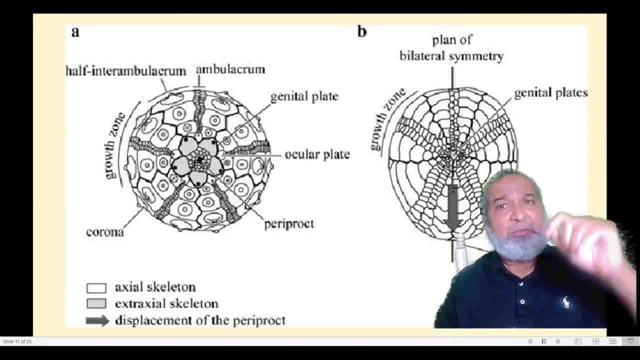 shape and whatever. the apical and peristome are not coming on the same line, so it is the irregular. so that is there Now. here, whatever we have, the three parts are there. first we will see the apical disk. the apical disk is made up of ten plates, apical plates which are there. they are the 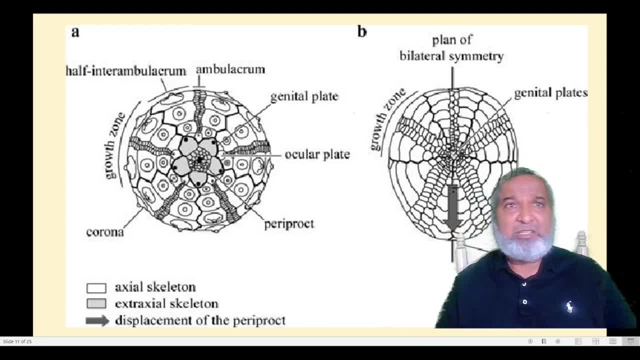 ten plates out of the ten plates. five are the bigger plates- these are called as the genital plates, and five are the smaller plates- that is called as the ocular plates, and the next one, the corona, which is there, which also contain the ten plates out of the ten. 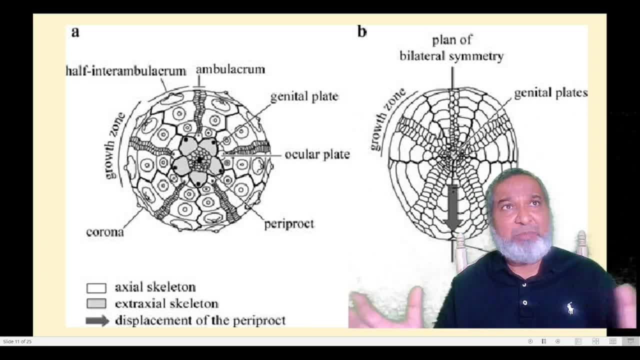 plates, five are a smaller one and five are the bigger. and between the two, bigger one, this is one and this is two. between this, whatever the dark line, what we have drawn, a small one. this is the ambilateral area and this is the interambulacular area, and 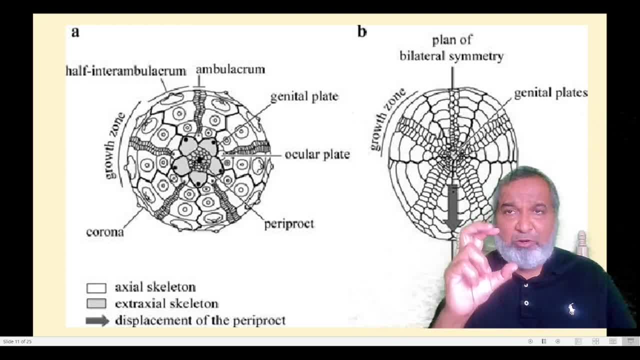 in this interambulacular area. we are going to see the rounded nodules. are there? nodes, are there from that nodes, spines is there? so to protect this animal? the spines are there. so should not? somebody should not be catch enemies, so the spines are there. 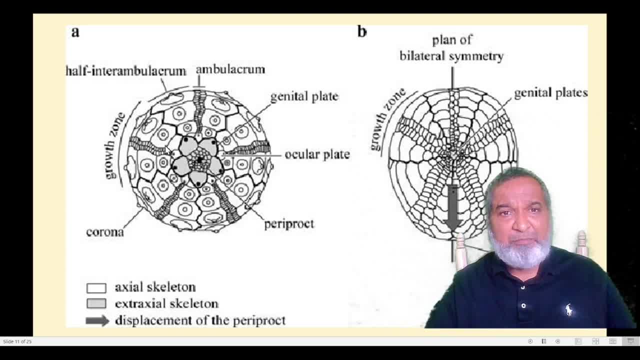 tubercles are there. these are there and these are the bigger one. so we have five ambulacular areas and five interambulacular areas. so the ten plates over there- these are the bigger one- then apical desk will be there, which is contained is also in the ten plates. you 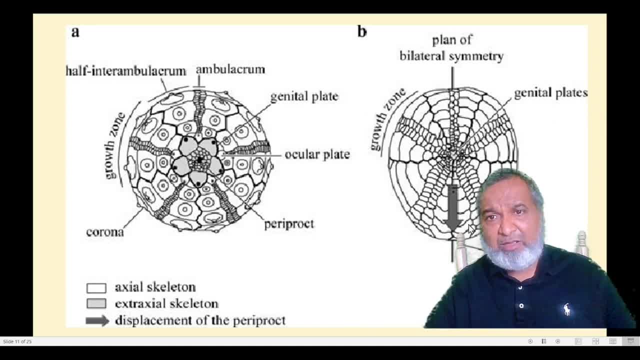 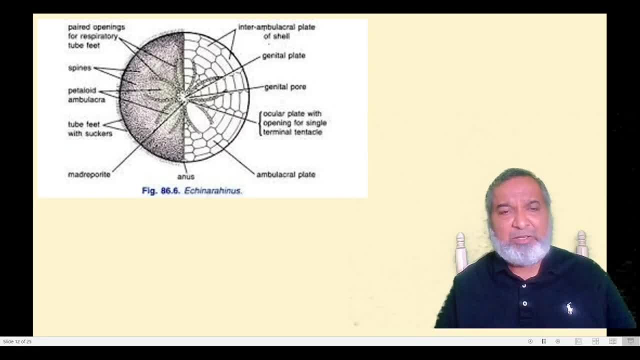 also can see: five are the smaller one and five are the bigger one. so these are what we have, the things which we are going to see, the same one, what we have shown, the diagram that has been made over here again repeat: the body is a. the tubercles are there. 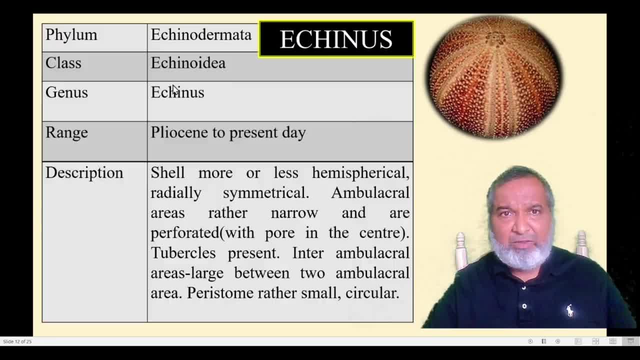 the rounded. what we have these are the tubercles. so so what we are? specimen. you can see this part which is there. tubes will be there, small one, See the round shoulder, as I mentioned. so this is the round shoulder, as I mentioned. 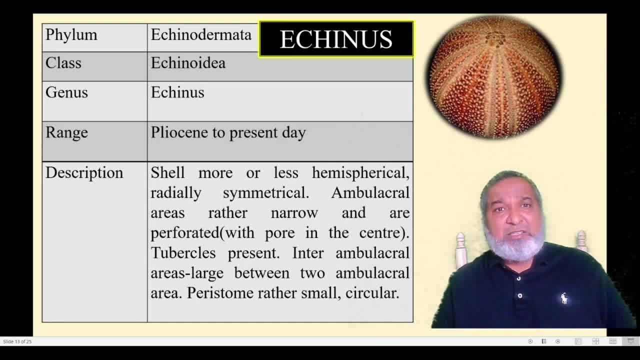 it is the round shoulder and this is the inner shoulder, and then, if you look at it from the Now, the first specimen is that Echinus, phylum Echinodermata, class Echinodea, and the genus is Echinus. 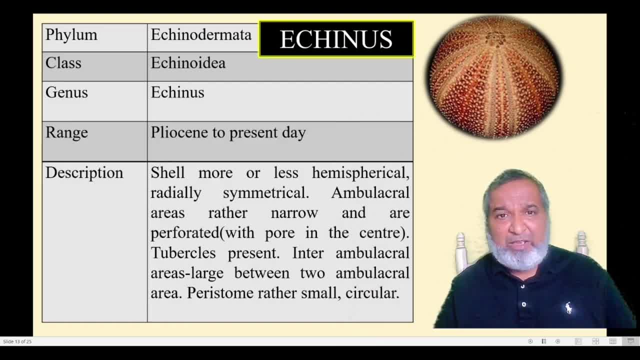 Pliocene to present it is there. Pliocene to the present scale is more or less hemispherical, radial symmetry, ambulocular area rather narrow and are perforated, that is tubercle present. interambulocular area, areas large between the two ambulocular areas and peristome rather 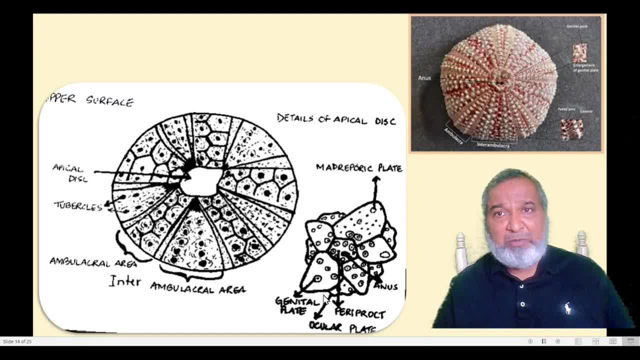 small and circular. So this is the part will be there and if you make out, this diagram is required. This is my diagram. I have drawn the diagram, the same diagram. you have to draw it out in the examination and you have to label it out. this one: 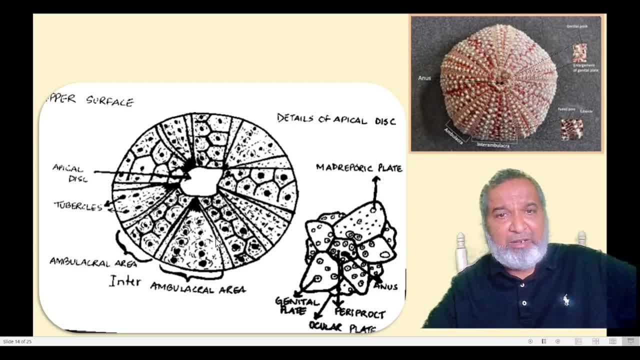 So 5 ambulocular areas and 5 interambulocular areas in the part of corona you have to draw, then the apical disc, then the templates. These are the templates and towards the anterior side, what we have, the genital plate, is a. 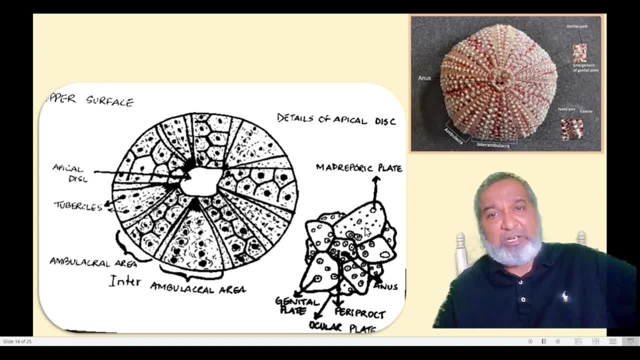 very bigger one And this plate is called as metriplegium. Yes, and the rest one. you can see 1,, 2, this is 3 and 4 and this is the 5th, so 5 we have. 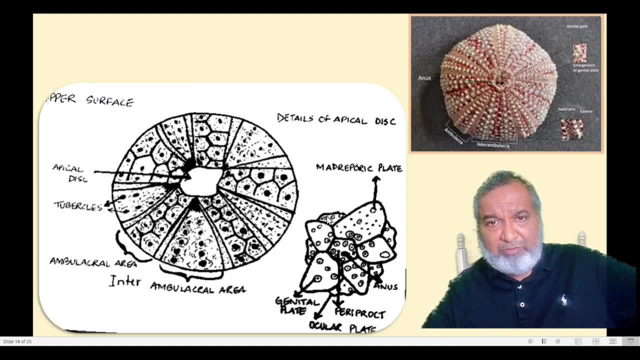 the genital plates and in between the two genital plates we have the alternate ocular plates are there. So if they are going to arrange side by side, then the insert and if exert also there. So these are short in the theory. it will ask that I am going to take it separately. 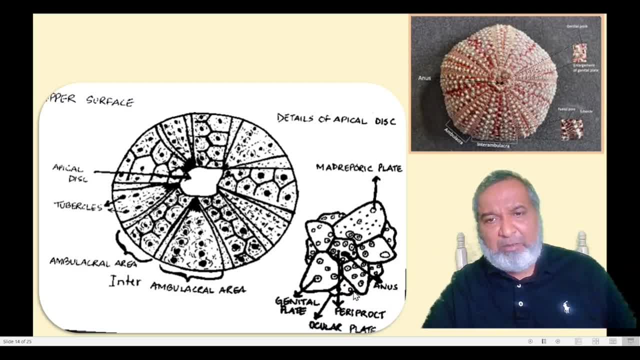 so no need to discuss here So that The part will be there. so the 5 genital plates, 5 ocular plates are there and in between we have the periproct is there, in that we are going to have the anus will be there and mouth. 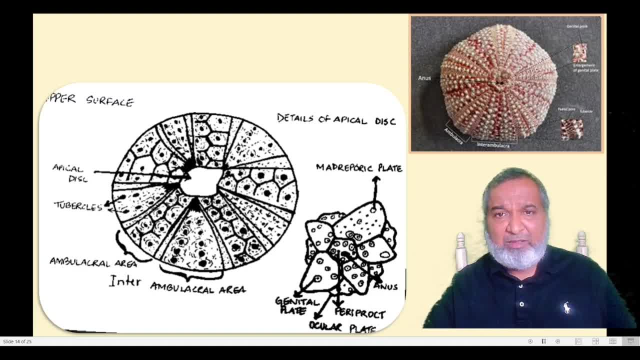 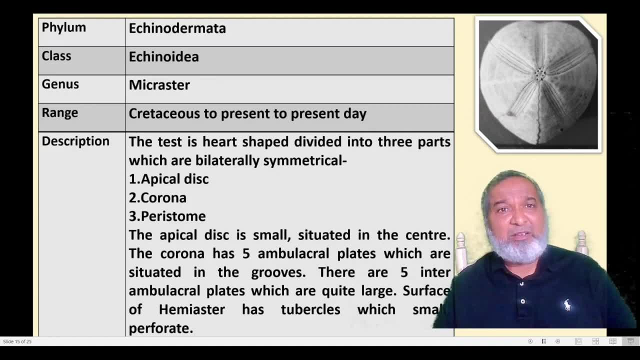 on the lower side. So this is what we have, the parts of this particular equinus, and the next one is equinodermata equinoidea and micraster. So here we are going to have a heart-shaped micraster from the irregularia. 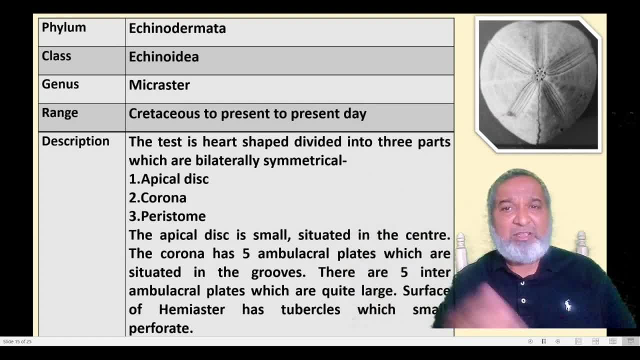 So if you make the subdivision over there in this, it will comes under the category of irregularia and it is cretaceous to present. yes, Again, there is a again spelling mistake is there? so again, cut and paste, So it is doubly repeated, so you can make out. cut out, so it should be a cretaceous. 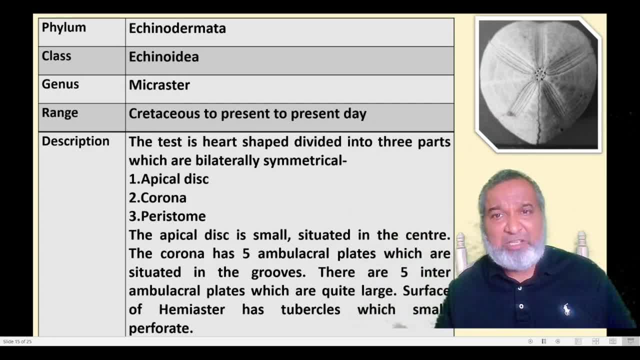 to present Now what is the description? is there test? is heart-shaped, divided into 3 parts: apical disc, corona and peristrome. apical disc is small. in this you can see now it is very small. It is situated in the centre. corona has 5 umbilical areas and 5 are the interumbilical. 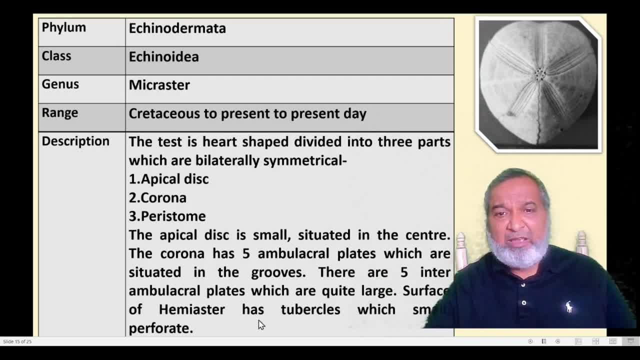 areas. So that will be there that we are going to cover, and hemiaster earlier one, we are taking the hemiaster but now hemiaster we are not taking, So tubercles will be there here. yes, cut and paste. this is again a problem. it should. 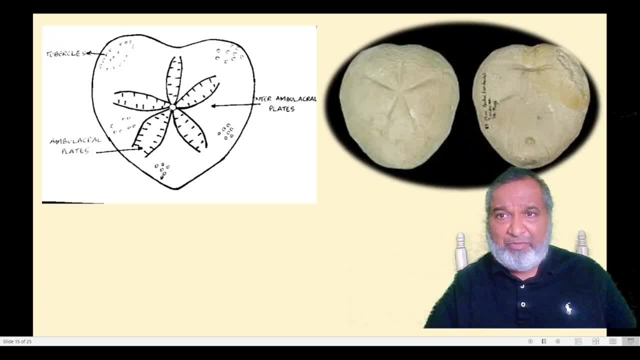 be a micraster one. the hemiaster is there. So wherever I am pointing out, we remember. now this is to be remembered. yes, here can have the fossa. Yes, this is a specimen hole in the centre and on the opposite side. so they are not. 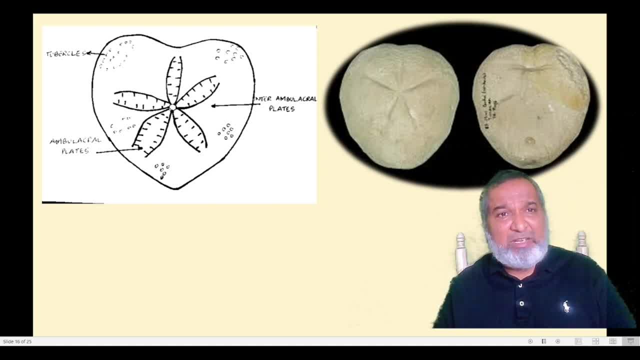 coming on the same one, So irregular area is there. that is why I told you this is the tubercles are there. see, this is what the tubercles will be there, and these are the 5 will be the umbilical. 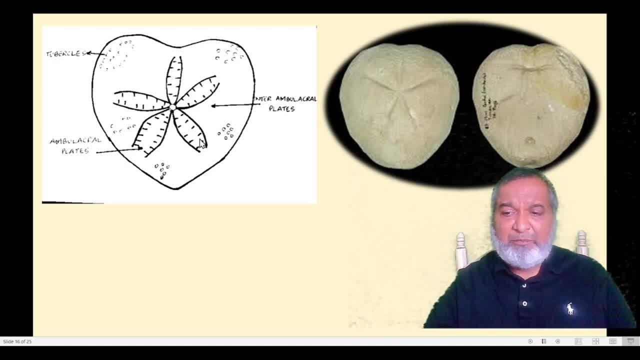 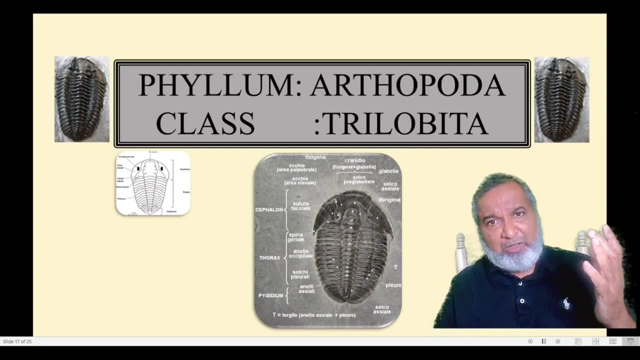 areas and 5 bigger interumbilical areas. So this is about what we have: the phylum Echinodermata, and in that we have seen the 2 specimens, Echinus, and the second one, Micraster. Yes, Yes, 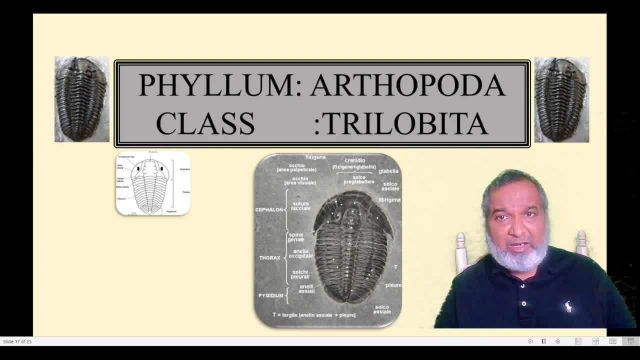 And the last one, the phylum Orthopoda and class Trilobita. So in this, what we have is the fossil, and here we have a lot of things. are there? yes, the body has been divided into 3 parts, horizontally as well as vertically. 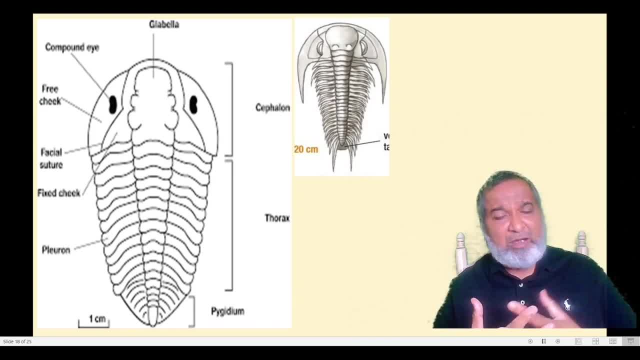 So this will be the quotient will be there in the theory. yes, I do not know now whether it will be there in the FY or SY, so that will be. there might be somewhere. it will be added parentology now. So the whatever the body is there body has been divided into 3, first upper part is a. 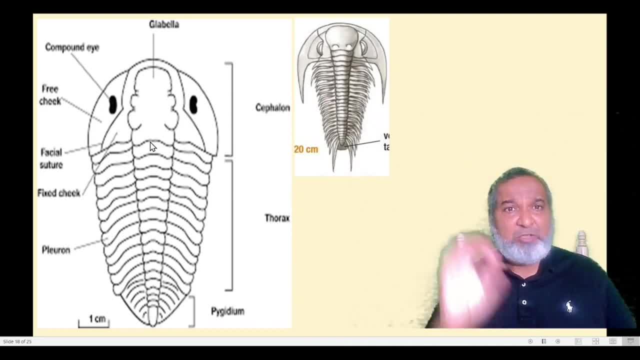 triangular. yes, it is a very hard exoskeleton. exoskeleton is there and that is called as a head or thorax- sorry, head or cephalon- and the middle part, somewhat a cylindrical in shape, is called as the thorax, and the last one, again a triangle, will be there. it is. 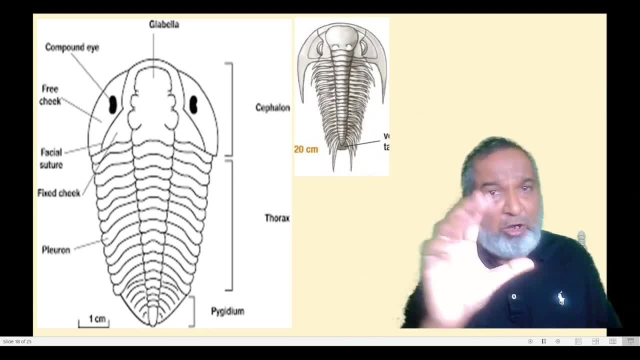 called as PgDM. So here the 2 triangles will be there, top and bottom, And the middle one is a cylinder. So this is the 3 parts which we have seen. the top is a triangle, one that is the head or cephalon, then the middle portion is a cylindrical one, thorax. next one in the lower. 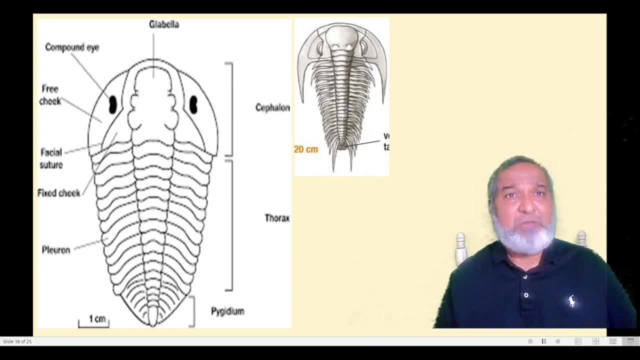 side we have again a triangle shape, is the PgDM. due to this horizontal division, Now I can make out the vertical division. if you have these 4 lines we have been drawn and due to this, now This is the divided into 3.. 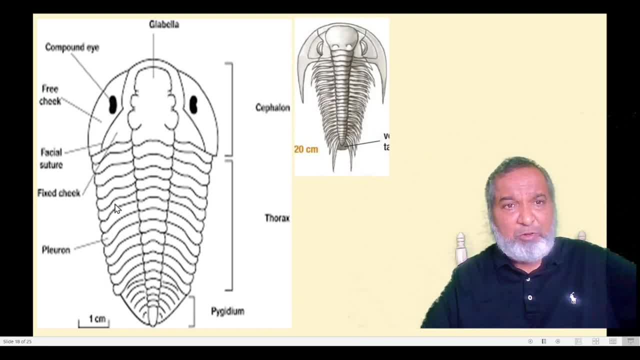 So what we have, the axial furrows and pural lobes. this is the pural lobes and axial lobes. So the body is divided into 3 parts and in that we have this, segments will be there, purons will be there and that will be the body will be there. 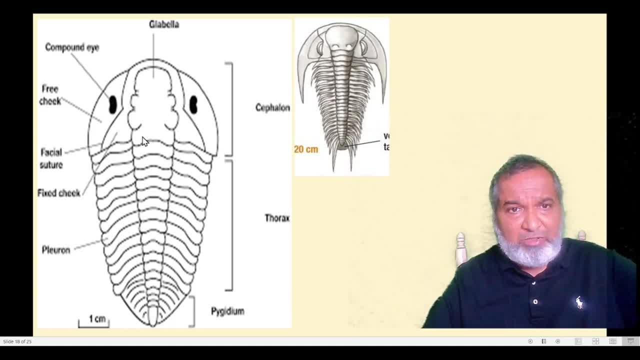 Now, one by one, you can make out here. say, now, only concentrate on this particular globula. there will be evolution in the globula. there will be evolution in the eyes. there will be evolution in the genital angle, that is, the genital angle is there and genital spines. 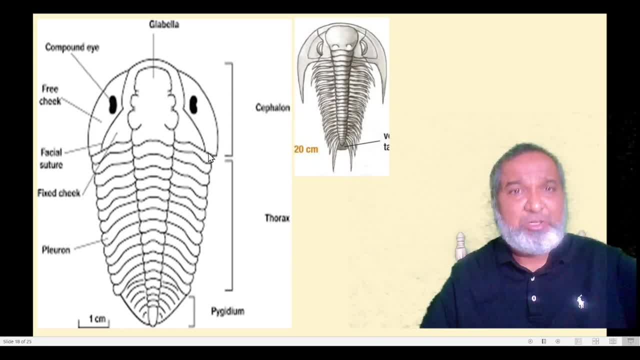 you are going to see now, this is the genital spine. so that is the evolution. in this eyes, evolution is there. So many evolutions are there. when you are going to see in the TY, there will be the evolutions that will be, the part will be there. so this is the globula. these are been like a shape. 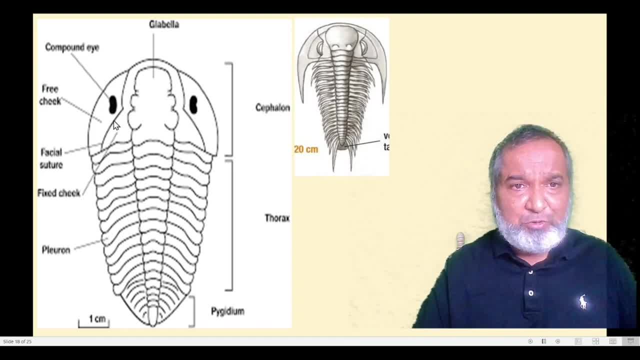 is the eyes are there. these are the facial sutures are there. this is the free cheek and fixed cheeks. These are there. then we have the. whatever the outline is there. it is smooth, segmented body is there and in this, segmented around, we have 25 to 45 segments, will be there in. 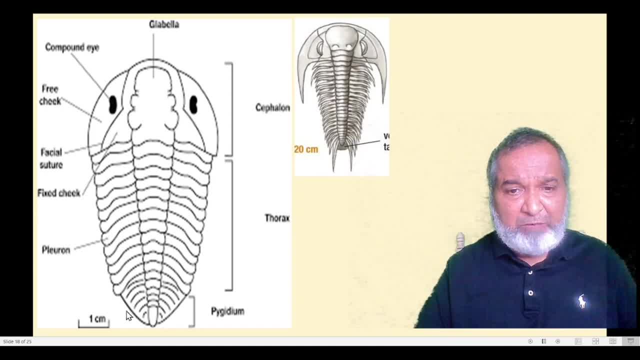 the thorax and around about 0 to 15 will be there in the PGDM and PGDM. sometime it will be smooth outside and, as you find out it will be. spines will be there. yes, one or maybe in two, number of spines will be there. that will be going to show you the variations. 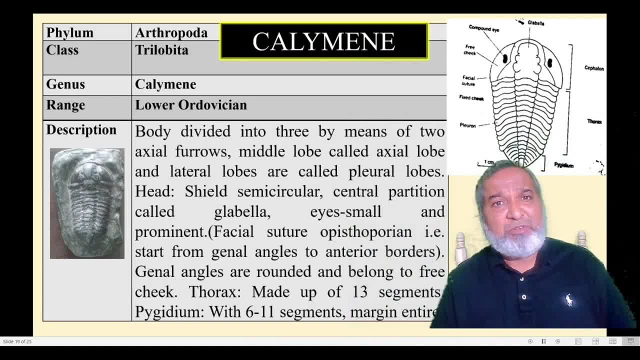 Now, in that the first one we are going to see, the casp fossil that is the casp, will be there. that is not a fossil casp, that is a calamine, that is a phylomerthoboda plus trilobita. 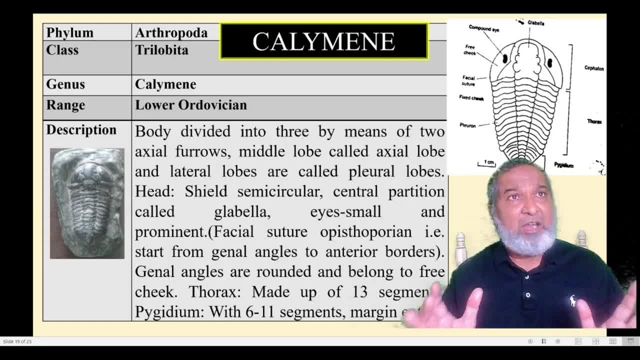 and the genus is calamine and it is extinct now lower odovician. that is why it is not easily available for fossil for our department and we are going to try it out. if you get it out, Then in the future batch we can show this particular specimen. 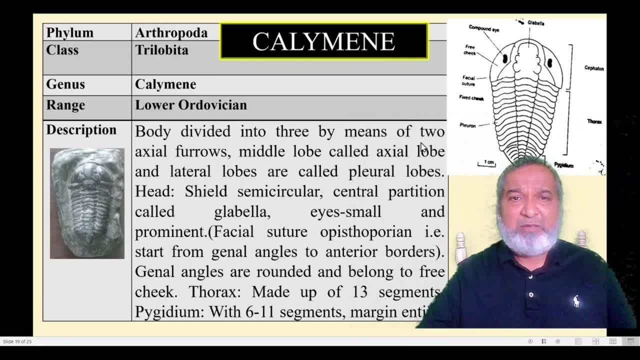 Thank you. So the body is divided into three means of two axial furrows. middle lobe is axial lobe and the lateral lobes are called as superior lobe. that we have seen. The head is semicircular. central portion is called as globula. eyes are small and prominent. 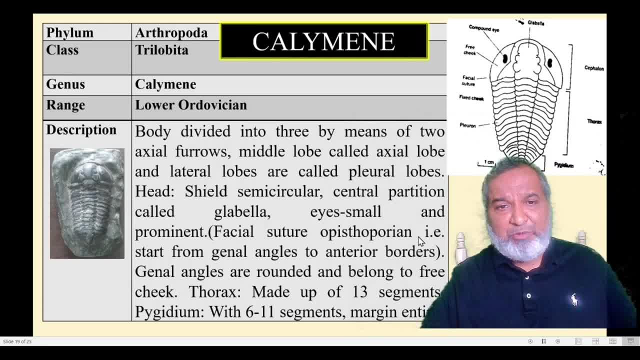 that is a bean shape. triceal suture, opto-polymeripodium start from the genital angle to the anterior body. Genital angles are rounded. yes, here, this is what we have. This is what we have. genital angle: this is the rounded one and belonging to the free. 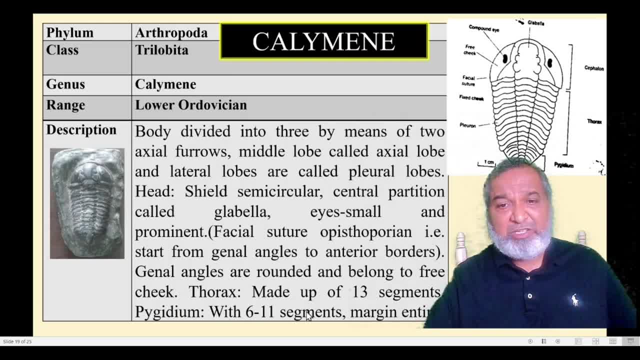 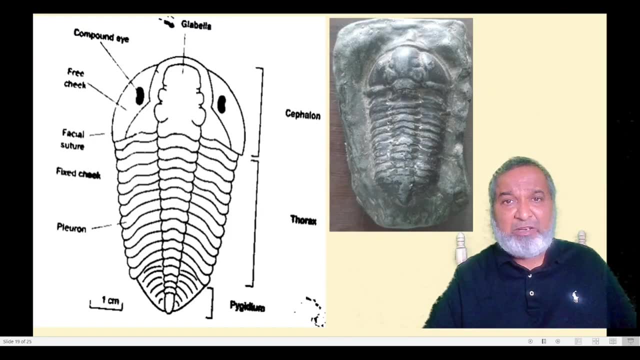 chicks thorax is made up of 13 segments. pgdm is 6 to 11, margin is entire. smooth margin is there, yes, and somewhere the middle part has been depressed and ultimately end. one part is there. Can see shape is a very interesting one when you are going to see that particular part. 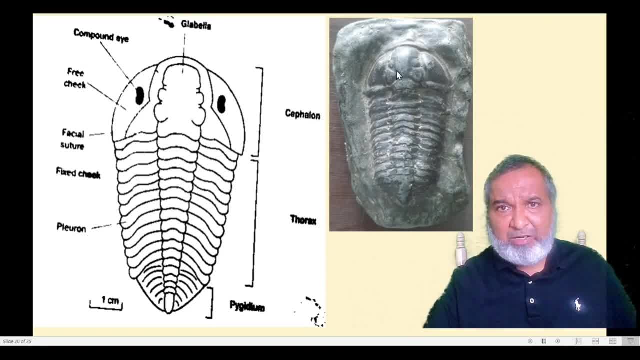 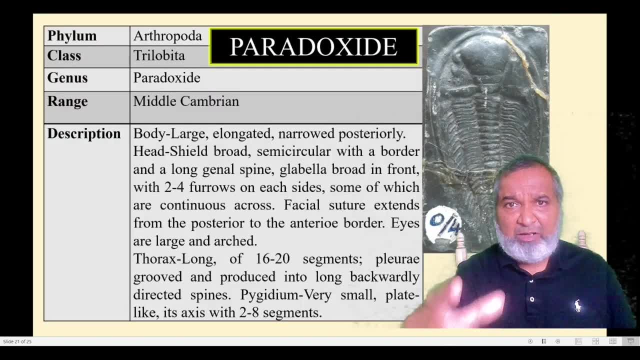 This is what we have, the fossil, with this particular diagram, you have to remember, because we have the two specimen we are going to take in the lab. This is one which is the calamine one and this is the peroxide. Now, peroxide, the outer margin is having the spines. genital angle is there? yes, very genital. 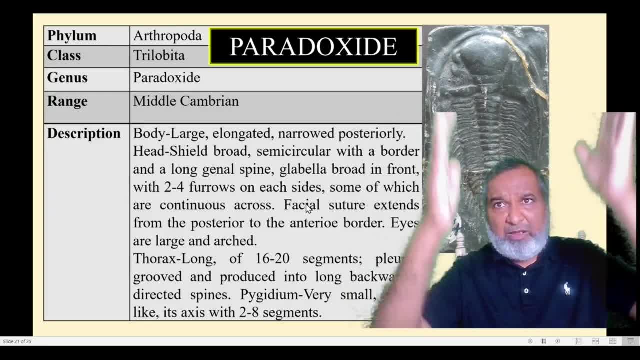 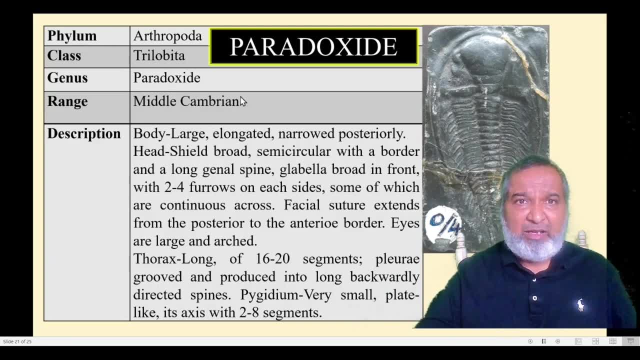 spine which is there globula, is very big. length is long and from the top it is go on becoming narrow towards the bottom. So it is a long body, is very large, as a length will be, as compared to what we have, the calamine. 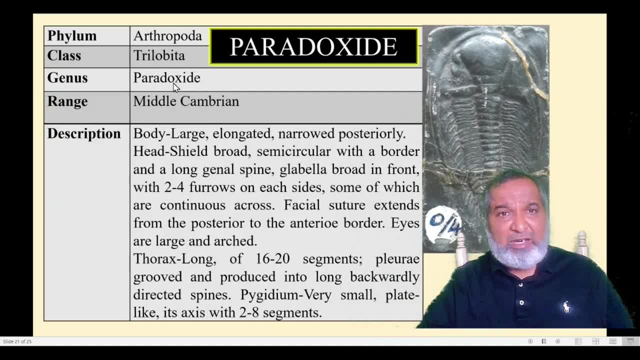 Stora class chrylobita, and genus paradoxite, and range is middle cambrian and body is large, elongated, narrow, posteriorly head shield, broad, semi circular, with the broad and a long genial spine, And sometimes the spines will be greater than the height. also, 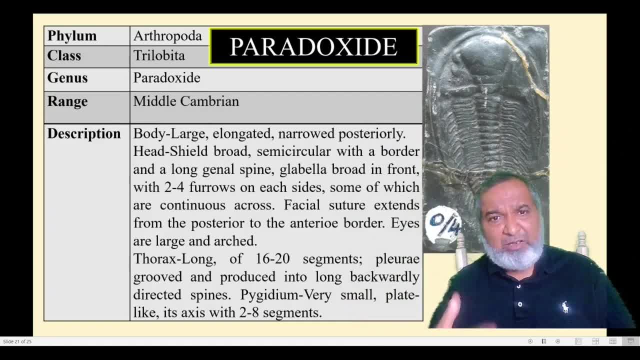 In some specimens what we have: genus there will be. spine will be greater than the height, also Globular, broad in the front, with the two or four furrows on each side. Yes, that will be there, but here they have not been shown. Faisal, suture extend from the posterior to anterior side. That is also not clear in this. 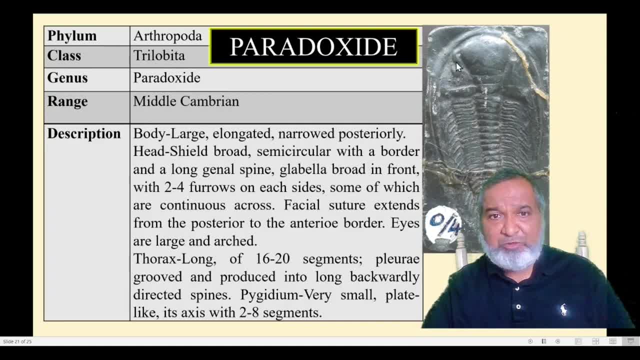 particular part. Eyes are large and you can see the eyes are shown as a large arch. Thorax will be 16 to 20 segments. Fura grooves and produced into long backwardly directed spines. So here we have the spiny outlines are there? Vision is very small and plate like it has two to eight. 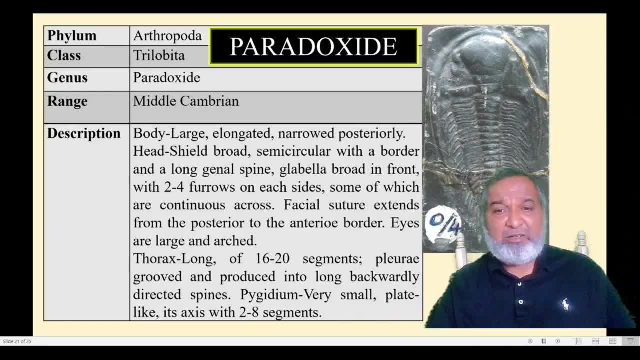 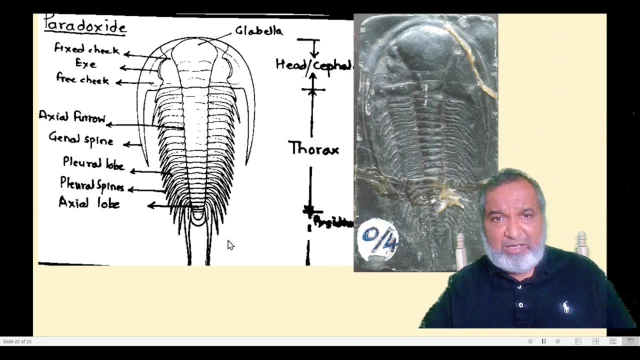 segments and there is a tail. is there? Yes, the tail will be present in that paradox side, but it is absent in the calumet. Yes, you can see now the same diagram I have been drawn. This is my diagram sketch- is there- So I could not get it time- so that I can make the scan Everything we can do it, But whatever we have, I have been drawing So I could not get it time so that I can make the scan. Everything we can do it, But whatever we have, I have been drawing So I could not get it time so that I can make the scan. Everything we can do it, But 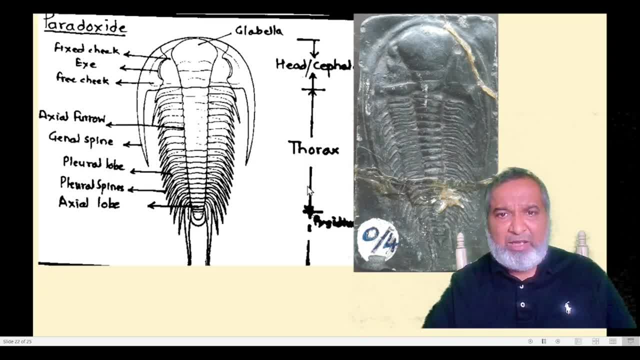 whatever we have, I have been drawing So I could not get it time so that I can make the scan Everything. we can do it, But try to show it out. what are the forms? head, thorax, frigidium, axial lobe, pural spine, pural lobe. 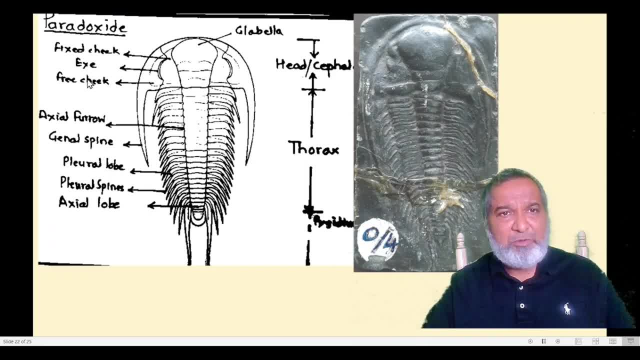 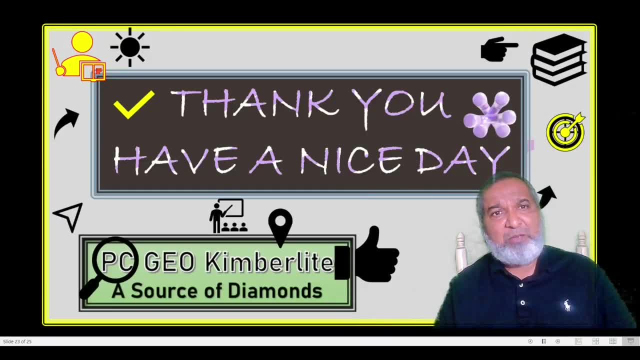 genal spine. Yes, that is axial foros, free check, eye fixed checks. So that will be shown whatever the specimens are there. With this we complete this second practical. that is small one because there are the three phylum, but there are the total. six specimens are there, But the whatever. 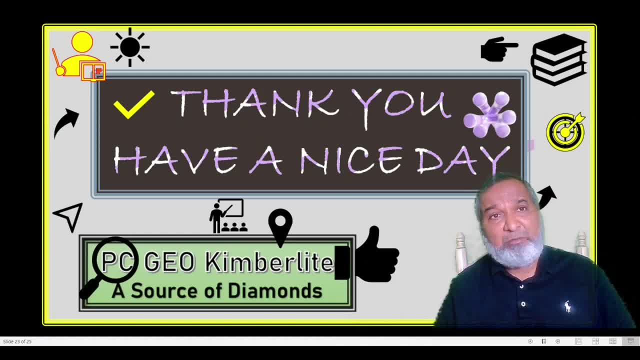 the background which is required. the erotical background is a very, very important one, whatever the parts which are there. If you know the parts very well, one or two times, if we go through this video, you will be remembering this. what are these parts of? that particular phylum is there and how to write this? 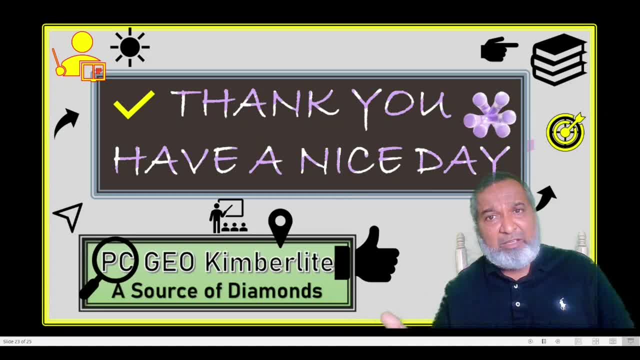 particular specimen in the examination, Because in the end, what is happening- this is a new subject, is that geology? and first time we have been attempting- and what to write, because before that we don't take any practical test, because we don't have a time to give you any revision. 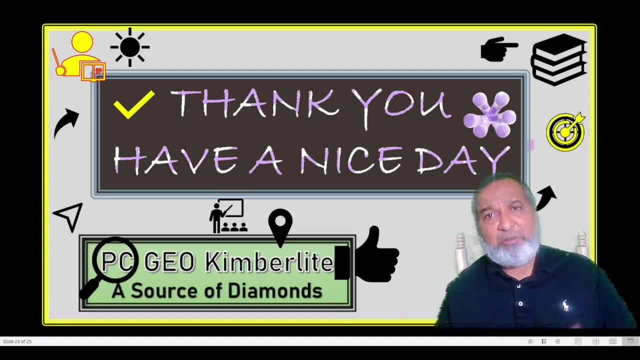 or we can conduct your pre-test. So that is not possible because of the short period of time is there and now it is a semester system. again, time is a very short one, So I don't think you can get a chance. but from my sides I am always telling the students so in the practical how to write.